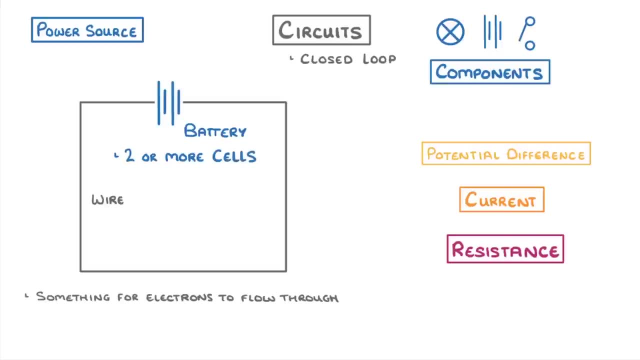 are made up of two or more cells, their symbol is just two cell symbols put together, Although as far as exams are concerned, cells and batteries act in the same way. Another common symbol is for the filament lamp, which is just a small light bulb. so 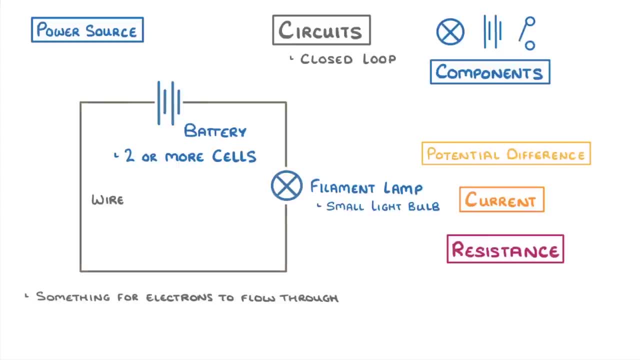 if we added one to our circuit and turned on the battery, then it would light up. We could also add a switch which could be closed, allowing current to continue flowing around the circuit, or open, which would disrupt our circuit and so turn off our light. 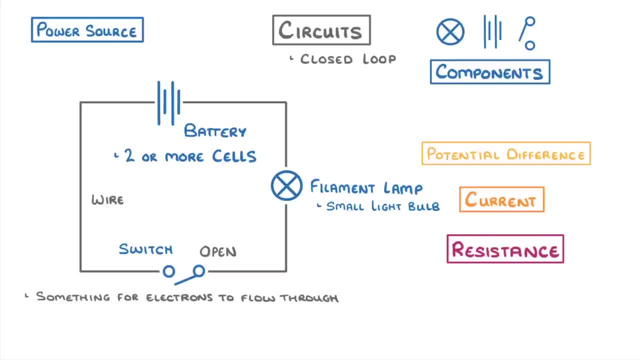 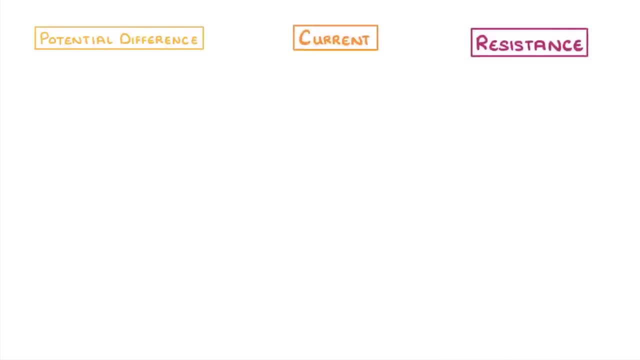 In order to explain what's going on, we need to look at some key terms, specifically potential difference, current and resistance. Current, denoted by the letter I, is a measure of the flow of electrons around the circuit, similar to the flow of water through a pipe, and it's measured in amperes. 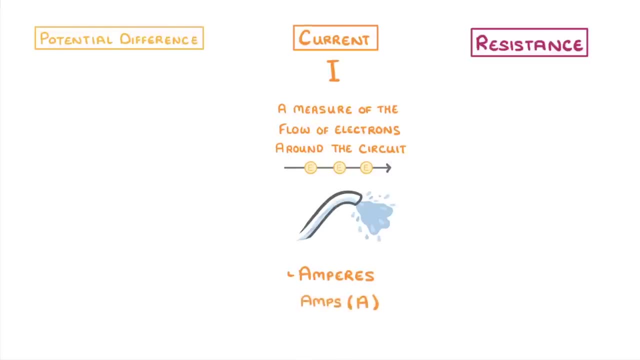 which are often just called amps and are denoted with the letter A. Meanwhile, the potential difference denoted by V is the force driving this flow of electrons and is provided by the cell or battery. You can think of this as the pump that forces the water. 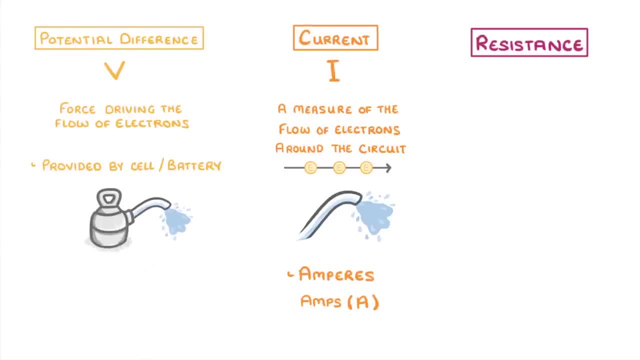 along the pipe. Another name for potential difference is voltage, and it's measured in volts Voltage. Finally, resistance R is exactly what the name suggests. It's everything that resists or opposes the flow of electrons, similar to a partial blockage in our pipe, example. 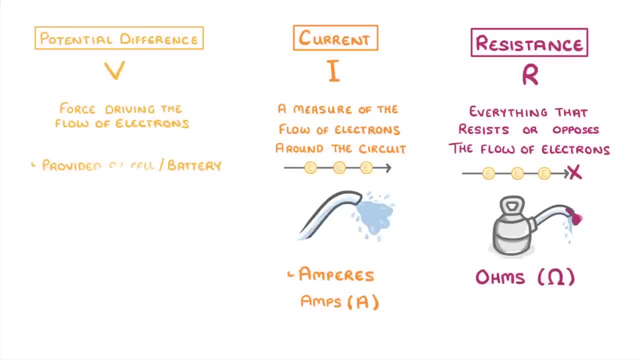 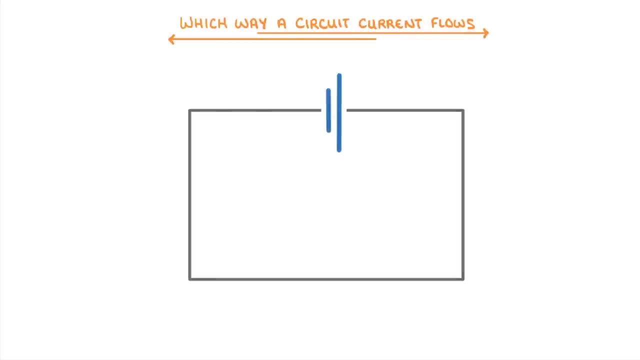 and it's measured in ohms. The last thing we need to cover is which way around a circuit current flows. If you look at the cell on this circuit diagram, you can see that it has one longer line and one shorter line. If you look at the cell on this circuit diagram, you can see that it has one longer line and one shorter line. 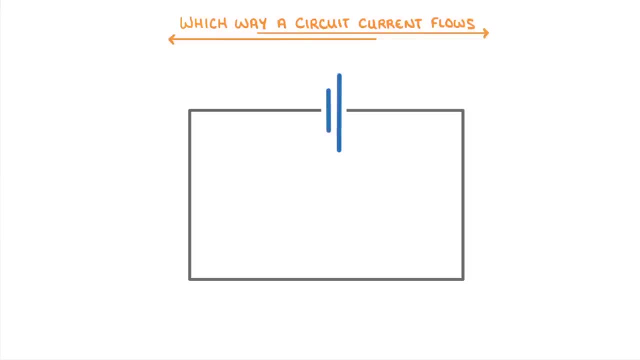 If you look at the cell on this circuit diagram, you can see that it has one longer line and one shorter line. The longer line in a cell or battery is always the positive terminal, whereas the shorter line is always the negative terminal.